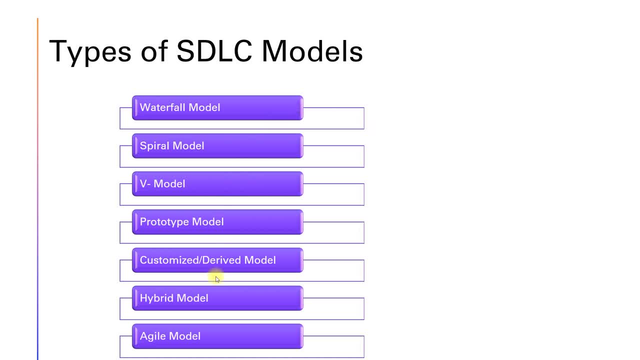 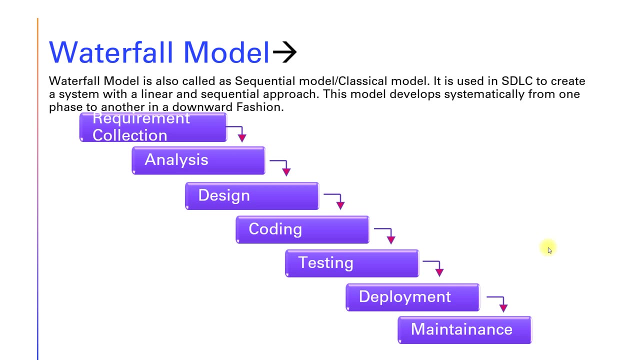 Okay, in this session we will discuss only six types of models: Agile model- I will take a separate class for this thing. agile model, because it's very important And with very featured. now Okay, what is waterfall model? So waterfall model is also called as sequential model or classical model. It is used in SDLC to create a system with a linear and sequential approach. This model develops systematically from one phase to another in a downward fashion. It is nothing just same as SDLC model. Your first is requirement collection, then is analyzation. 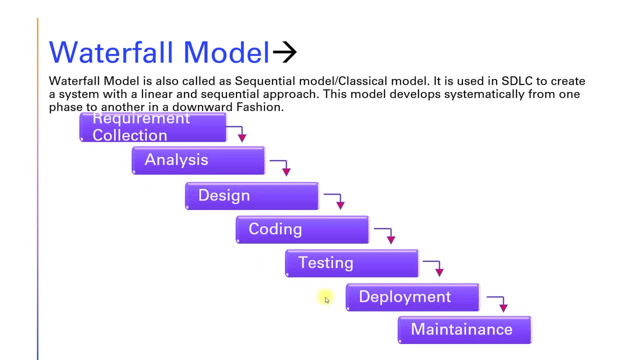 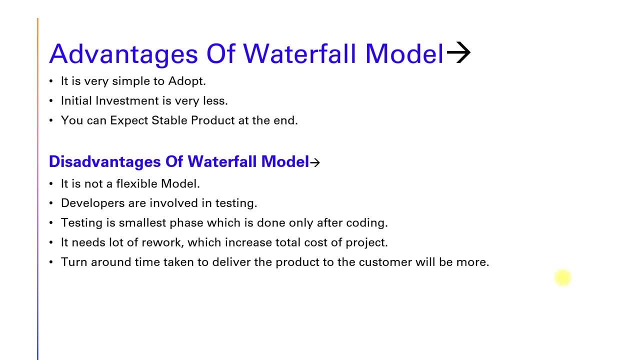 then design, then coding, then testing, then deployment and then maintenance. advantages of waterfall model. so what is the advantage? it is very simple to adopt. initial investment is very less and you can expect a stable product at the end. so this advantage is like it is not a flexible model. developers are involved. 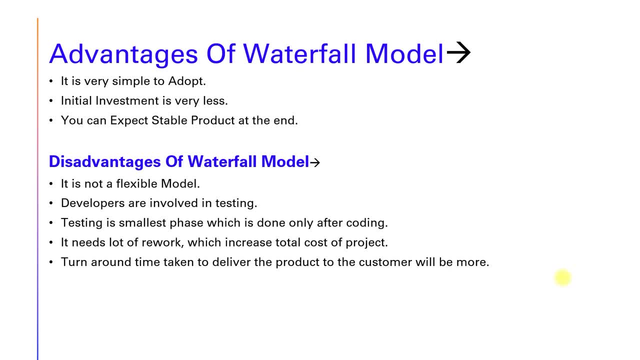 in testing. testing is smallest phase which is done only after coding. it needs lot of free work which increase total cost of project turnaround. time taking to deliver the product to the customer will be more one by one. we will understand. okay. so what is first? it is like it is very simple to adopt because 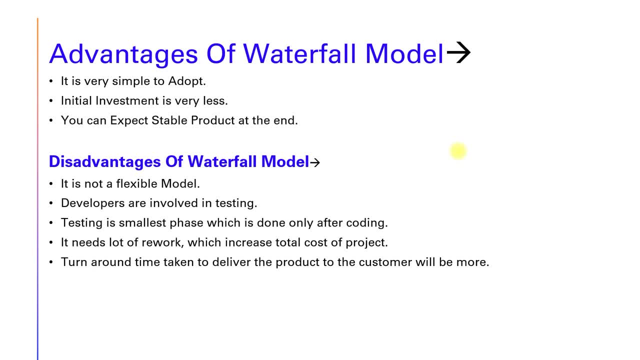 it's like: first is a requirement, collection analysis, then your design coding. thank you for watching and if you like my video, pls subscribe". testing, deployment and maintenance. so that's why it's very simple and initial investment is very less. so we are not doing any proper planning for that, so only we can estimate: yeah, such amount is. 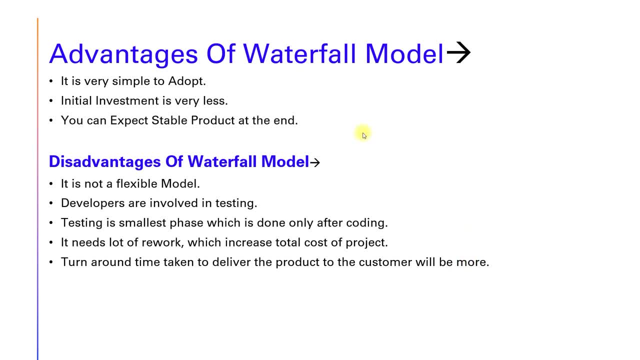 needed. so maybe like that then you can expect stable product at the end. because if, because requirements were freeze in the beginning, only okay, you must have some questions on your mind that why they will freeze the requirement, okay. so if there is any changes in the requirement at 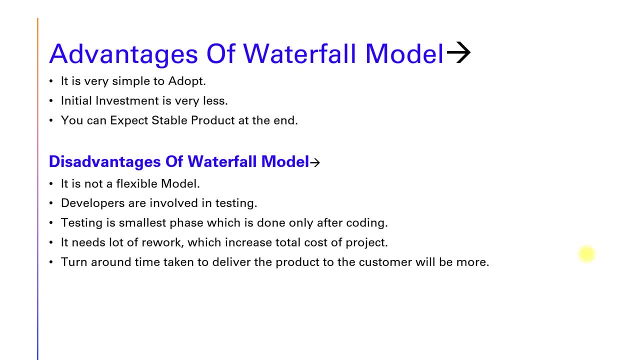 any stage then that corresponding design also changes. as the design changes, codes also changes. because of this, lots of bug will introduce in the code. to avoid all the above, they will freeze the requirement, okay, and the next question is that why they will keep changing on their requirement. so what happens? 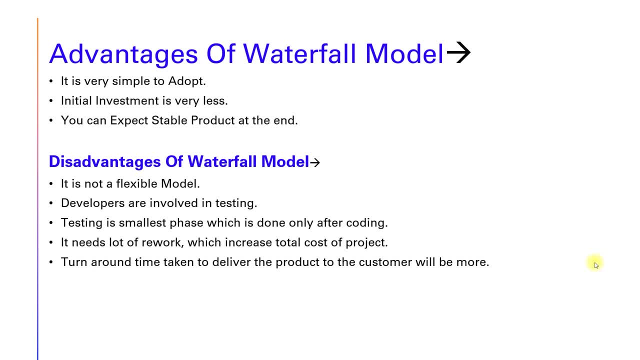 actually, every software supports business and business gives on changing, when the business chains- that's of a support software- should also be changed and also to adopt new technology, did they keep changing the requirement? so next is: like developers are involved in testing, what is the disadvantage? so if developers are involved in testing, what are the? 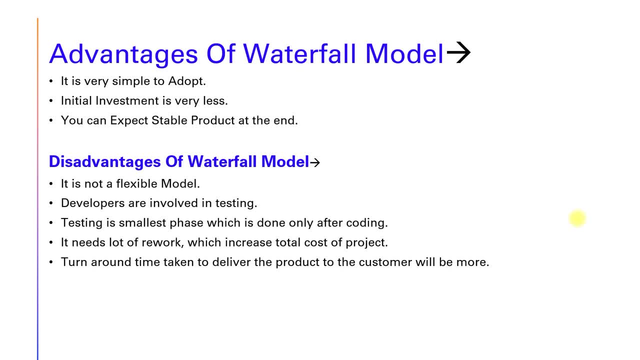 drawbacks let's discuss. so what will happen? they will not see their product from the negative point of view. okay, so they somehow want to build a product. they don't want to see the product breaking and they consume all the time allocated for testing to build the product and finally they say there is no. 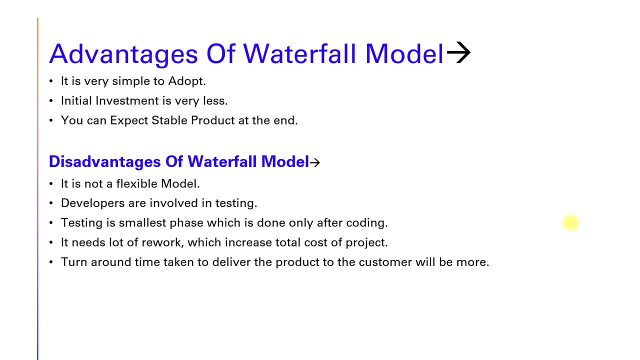 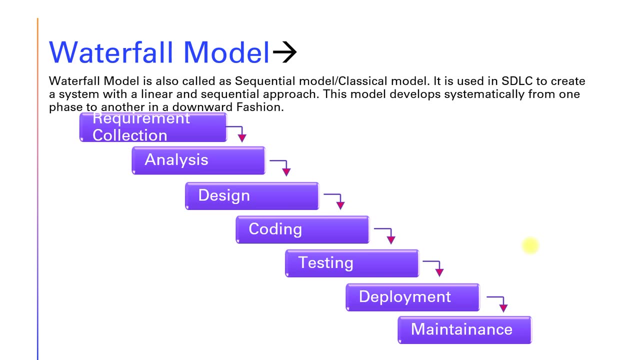 time for testing. and then what will? they will try to hide the box instead of fixing the bugs. so these are the advantage, this advantage. ok, then we will discuss about what are the applications of waterfall model. ok, so what is the application like when we build shorter or simple application? 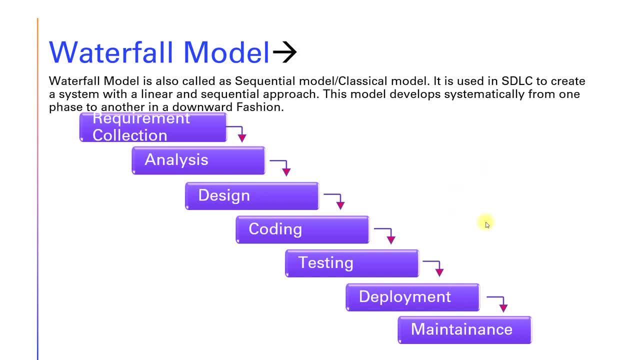 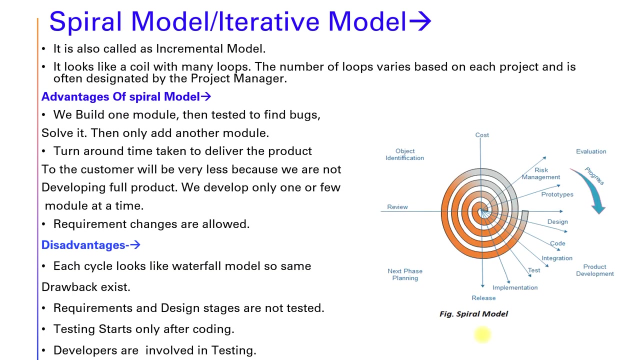 then we go for waterfall model. then second is like: when we go for short term project, then also we can adopt that waterfall model. then third is like when we have a short term work space, вот like keep Rs and we will create and create 애 wrap. so what is the Main or Second اس of water? 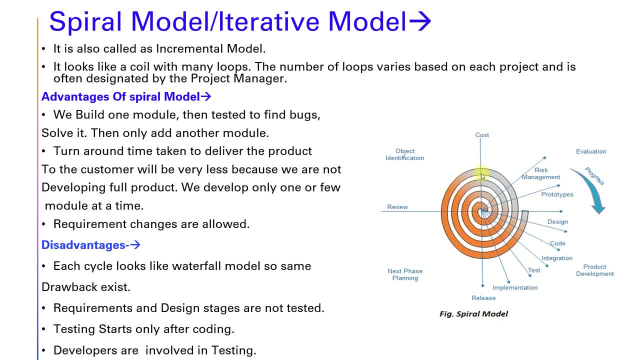 roll model. we have separate issues. what are theGuns? do you want to build simular model of water roll model? See how it looks like. It looks like a coil with many loops. The number of loops varies based on each project and is often designated by the project manager. It is same like waterfall model. It works like waterfall model. 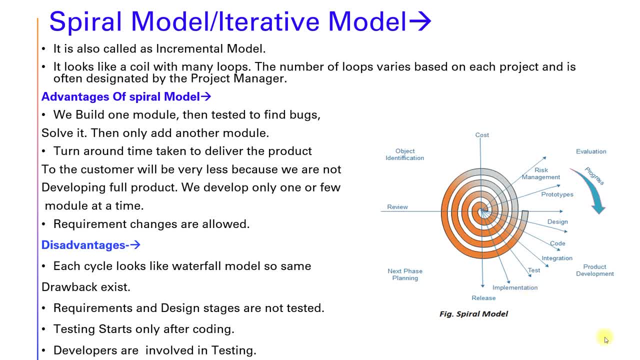 Advantages of spiral model. So what is happening here? First advantage is like we: first we build one module, then test it to find bugs, then solve it, Then only add another module. Okay, So that what happens? turnaround time taken to deliver the product to the customer will be very less. 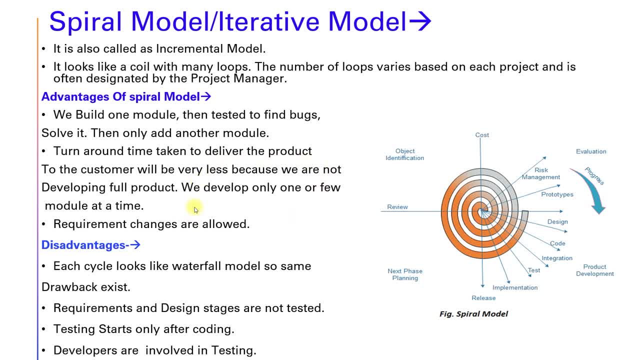 Because we are not developing full product. We develop only one or few module at a time. So so that requirement changes are also allowed When we go for spiral model. Okay. So whenever there is a dependency between modules and when requirements are given in stages, then only we go for spiral model. So it's disadvantage is it each? 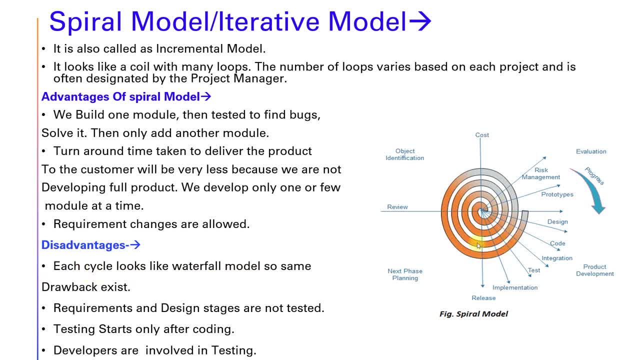 show cycle looks like waterfall model. So same: first is like your requirement, and then analyze, then design, coding, testing, deployment. So it's same thing, same like a waterfall model. and requirement and design stages are not tested. Testing starts only after coding and developers are involved in testing. So these are the disadvantages. 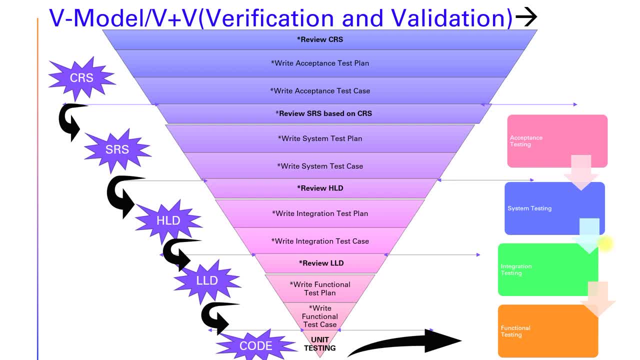 Then is B model. What is we model? that is verification and validation. So what is B model? B model: Why it used: in order to overcome the drawback which was there in waterfall model. we can move with B model. Okay, First how it works like. first is CRS. What is CRS? 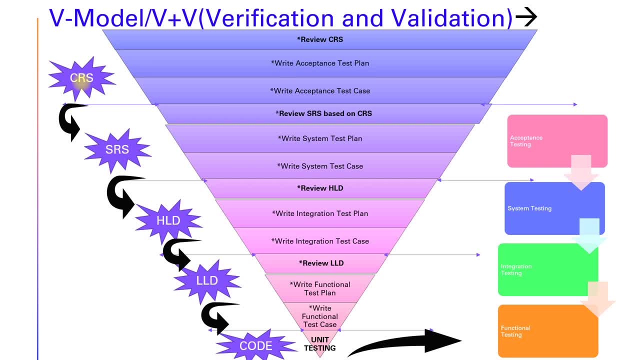 CRS is like customer requirement specification. okay, so here in the beginning, only your business analyst, product analyst and your QA lead or your manager or developer. they will meet and they will sit together and they will discuss what after that, what they will do. they will convert CRS to SRS. scared, his is like customer requirement specification and SRS is like. 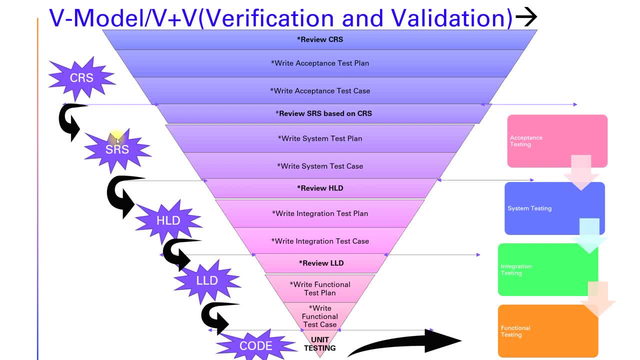 software requirement specification. what they did. their first customer requires is specification to customer requirements, specification to software requirements specification. at the same time, what in the QA team I mean, yeah, the testers, what they did, did, do, they will do. do they just review CRS, then write acceptance test plan and then write acceptance test case? 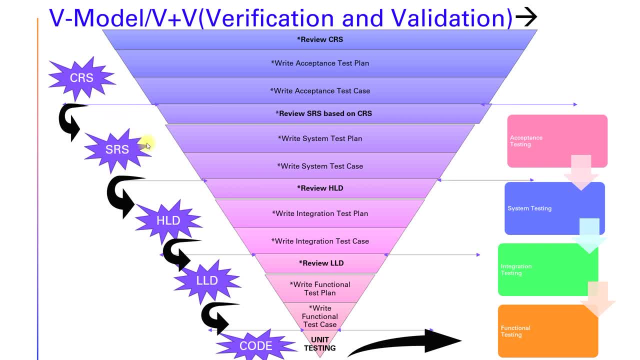 ok, based on CRS. ok, then what will they do in SRS software requirements specification? so they will review SRS based on CRS, write system test plan, then write system test case. ok, after that SRS will convert to HLD- high level design- ok. so then what the testing team? 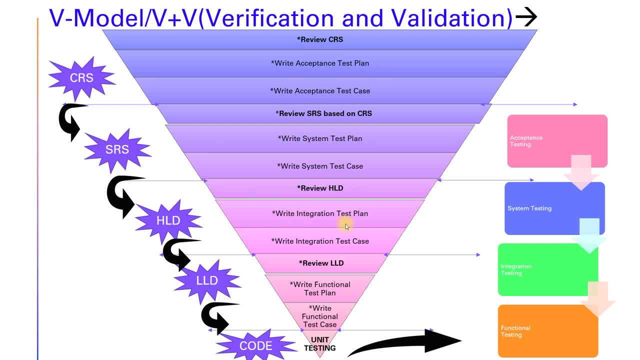 will do? they will do: review HLD, write integration test plan, write integration test case. then HLD will convert to LLD- low level design. so at the same time, what they will do like: review LLD, write functional test plan, write functional test cases. then starts test. 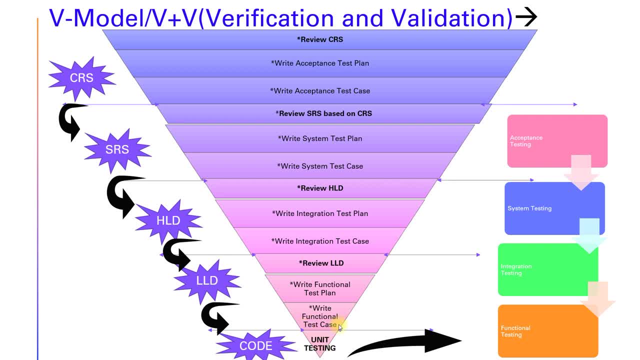 coding what, which is nothing, called as unit testing, or sometimes it is called as white box testing. so after that, here all QA team will involve testing team and they will start functional testing. then, based on their functional test plan and functional test cases, they will do functional testing. then they will, after functional testing, they will do integration. 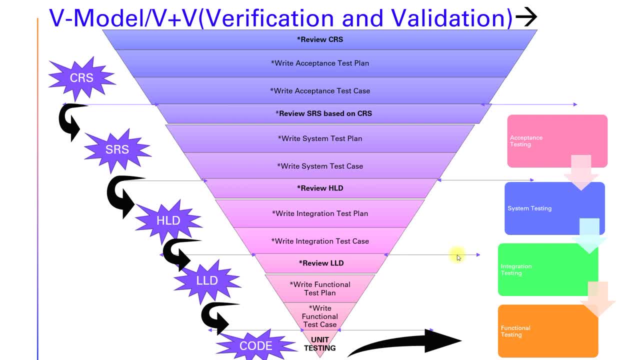 testing based on integration test plan and test cases. then they will do system testing based on system test plan and system test case. then, at last line, the last, they will do acceptance testing based on acceptance test case and acceptance test plan. ok, that is complete V model. how it this? how that V model works? so now discuss about. 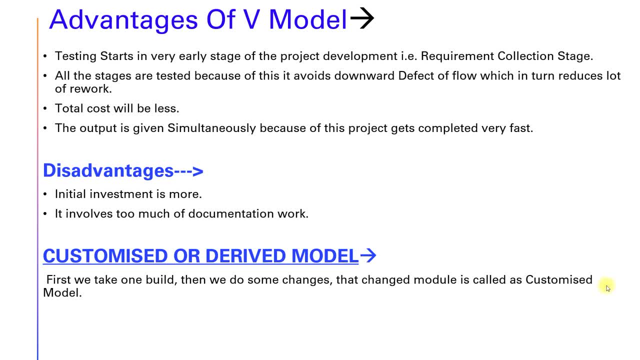 advantage, of advantage of V model model. so for what is the advantage? so testing starts in very early stage of the project development, that is, requirement collection stage. so all the stages are tested. because of this it average downward effects of flow, which is turn reduces, which in turn reduces. 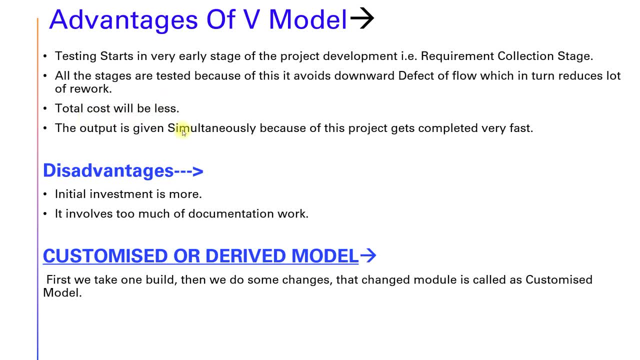 lot of rework, so total cost will be less. the output is given simultaneously. because of this project get completed very fast. so when we go for v-model, ok, so it's like applications. so when we build complex or larger application, then we go for v-model, and when we go for 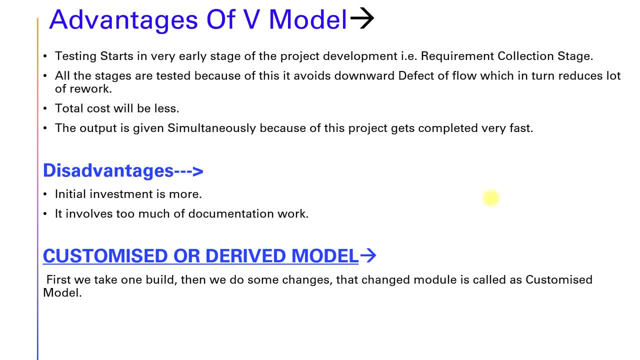 long term projects or when customer is expecting very high quality product under high time frame, then we go for v-model. and what are the this advantage? its first is: initial investment is more and it involves too much of documentation. work then is like customized or derived model. so what is customized model? it is nothing. 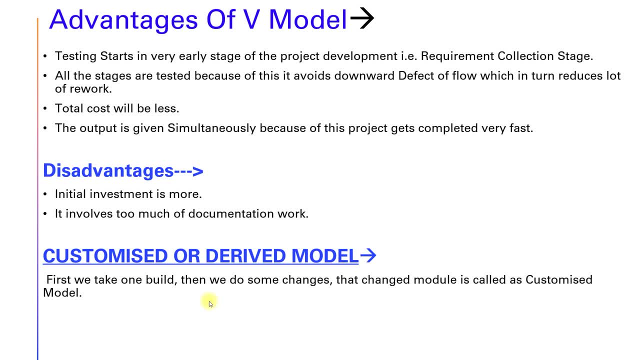 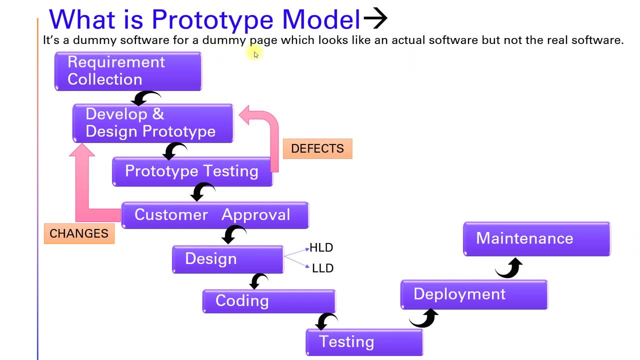 like: first we take one build, then what will we do? we do some changes and that changed module is called as customized model. then comes to what is prototype model? so what is prototype model? it is a dummy software or dummy page which looks and which looks like an actual software, but not the real software. 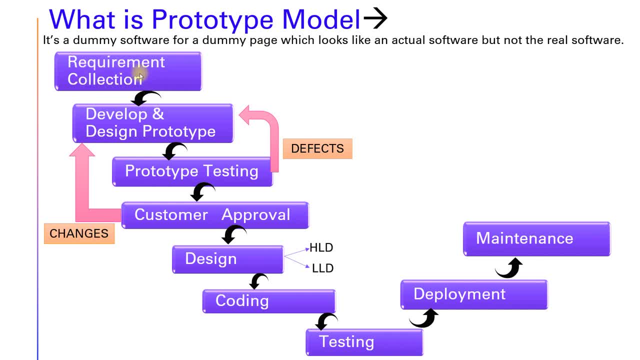 ok, so it like it looks like first is same thing like: first requirement collection, then development, design prototype, then prototype testing, then customer approval, design HLD or LLD, then coding, then testing deployment, maintenance. then customer approval, design HLD or LLD, thencoding, then testing, deployment. 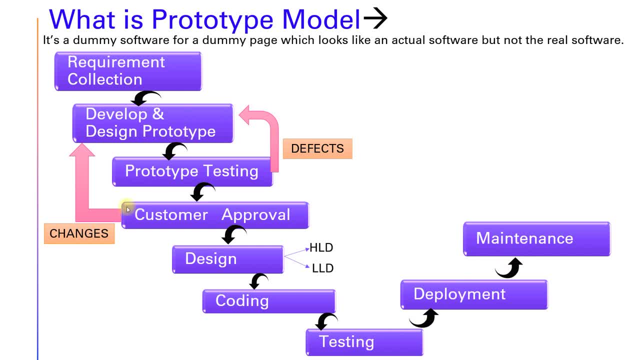 maintenance: okay, here, what is happening? one more thing is here is customer approval here, okay. so if there is, uh, any defect, first is requirement collection: okay, they will gather some. what is the requirements? then development and the design prototype: what will here? they will do, they will. 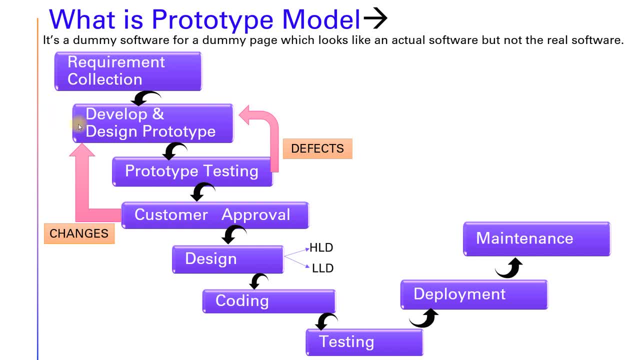 do text format to image format. they will change that requirement too. then what the prototype testing? prototypes testing is like: uh, they will test that features are present or not, features are, um, features are present at right place or not, and look and feel of the application. okay, he, then this page they will test. if there is any defects, then what will happen? they will. 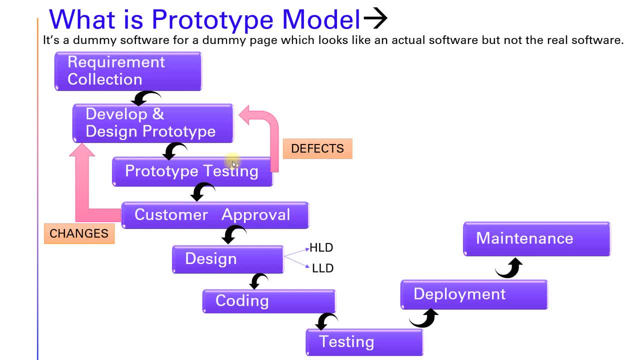 back to development and design prototype. okay, if, uh, it, it, this design will apply by customer. if there is an customer approval or customer will approve, then then it will go for design, coding, testing, deployment and maintenance. okay, if customer want to change some requirement or something, some changes, then what will happen? it will back to 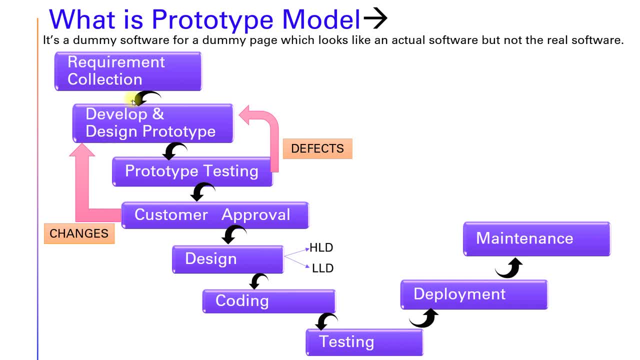 develop and design prototype. okay, this is how it works. okay, when we go for prototype model, okay. so, when customer is not clear about explaining his own requirements, okay, then okay. and another case is when customer is new to the software development process and also when developers are new to the domain, okay, 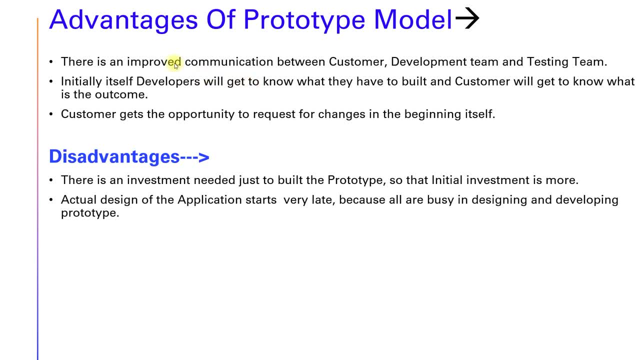 then we will discuss about the advantage. okay, what are the advantages? this: there is an improved between customer development team and testing team. initially itself, developers will get to know what they have to build and customer will get to know that. what is the outcome? okay, customer also gets the opportunity to request for changes in the beginning itself. so now discuss. 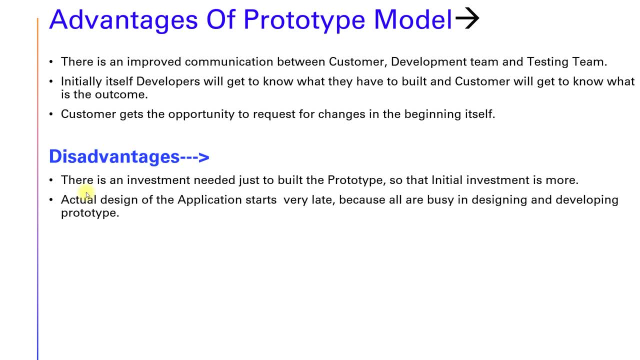 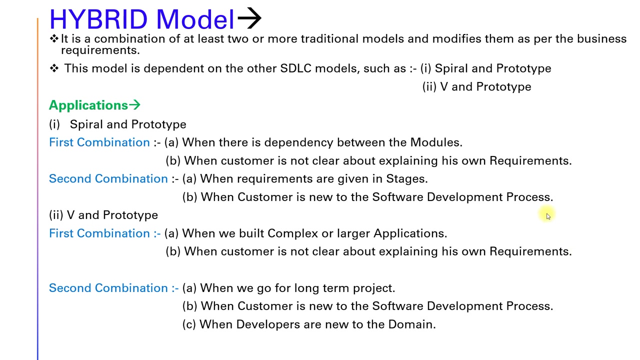 about drawback. okay, so first is like there is an investment needed just to build a prototype. so that investment issue, that the initial investment is more actual design of the application, starts very late because all are busy in designing and developing prototype. well, last we will discuss about hybrid model. so it is a combination of at least two or more traditional models and 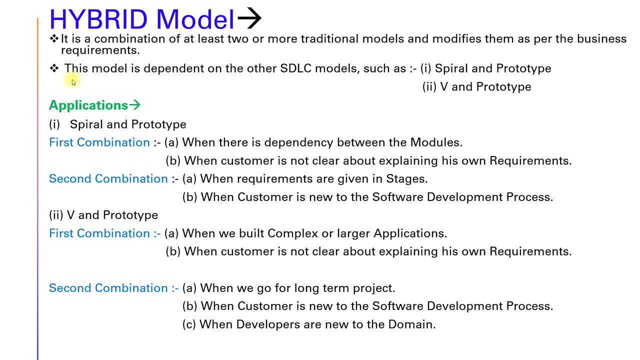 modifies them as per the business requirements. the this model is dependent on the other stl models, such as spiral and prototype, or v and prototype or spiral and way you can. you can combine any two models. so i have combined like spiral and prototype. okay, the first combination is: uh, what is the application like when we go for hybrid, hybrid model? so when there 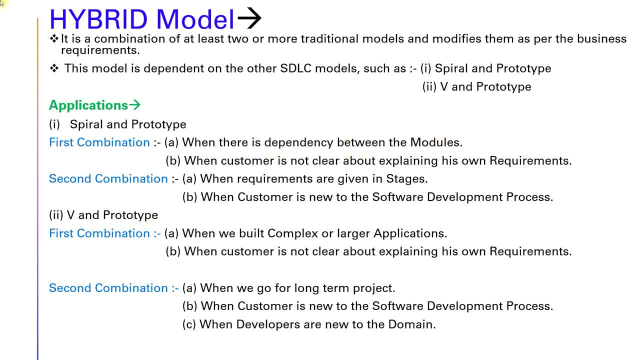 is dependency between the modules and when customer is not clear about explaining his own requirements. and second combination is like when requirements are given in stages and when customer is new to the software development process, and okay. then second is like v and prototype. so here is the first combination is like when we 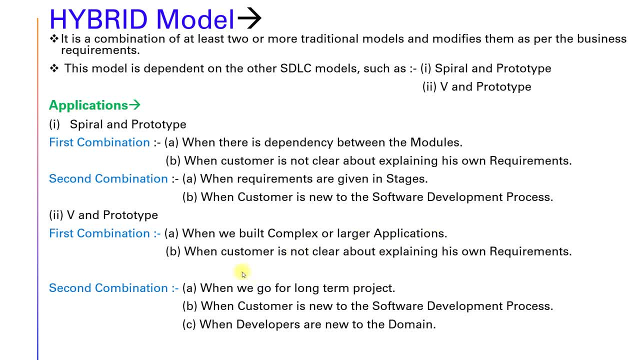 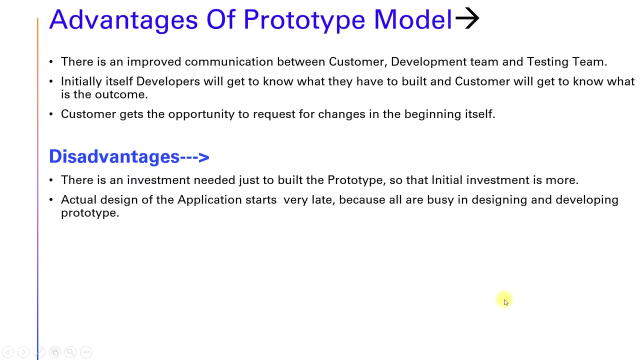 built complex or larger application. and second is when customer is not clear about explaining his own requirements. okay then. second combination is like: when we go for long term project and when customer is new to the software development process and also when developers are new to the domain, then we will go for hybrid model, then for agile model. i will take separate session for 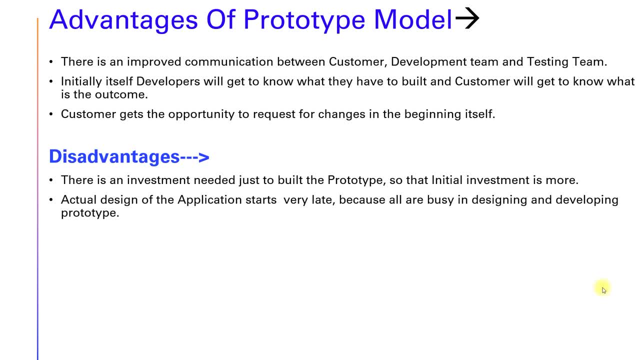 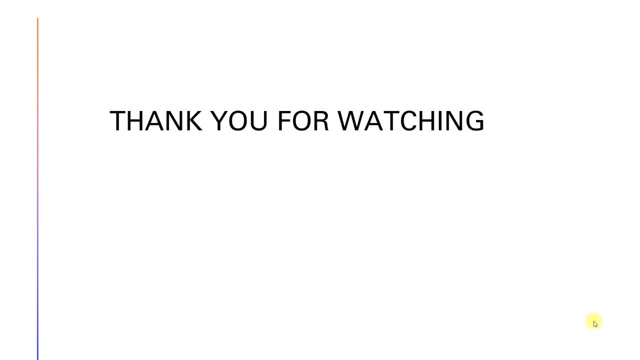 that okay, so in the next session we will discuss about software development testing. till then, thanks for watching and please don't forget to subscribe, like and share my channel. thank you.